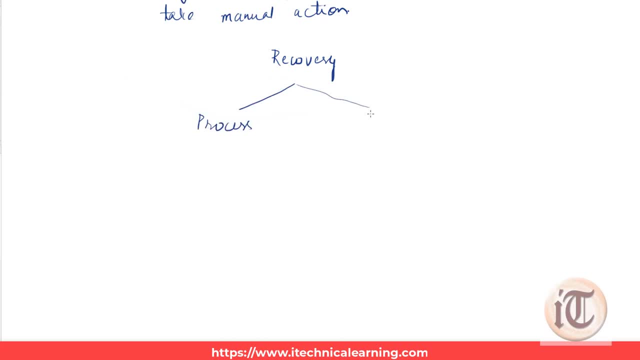 which it can perform the deadlock recovery. that is processes or resources. okay, so there are two basic approaches to deal with the processes. so this processes dealing is generally called as terminating the processes. okay, so this terminating process can have can be done in two ways, that is, kill one and second is called as kill all. okay, so kill one. 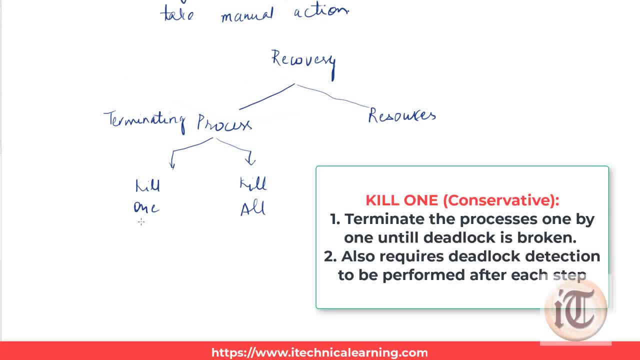 approach says that terminate the processes one by one until the deadlock is broken. okay, so, as you can see, we have to identify that which process is going to be terminated next. so this approach is more conservative, okay, but it also requires deadlock detection to be performed after each step. okay, and the selection of processes on which we 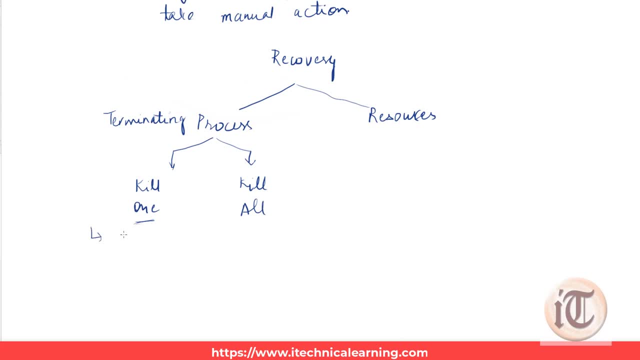 identify that this process will be deleted or terminated may be the priority. that, on the basis of the deadlock process, will be deleted or terminated may be the priority. that, on the basis of the process, will be the priority we can identify. maybe the execution time, maybe the number of. 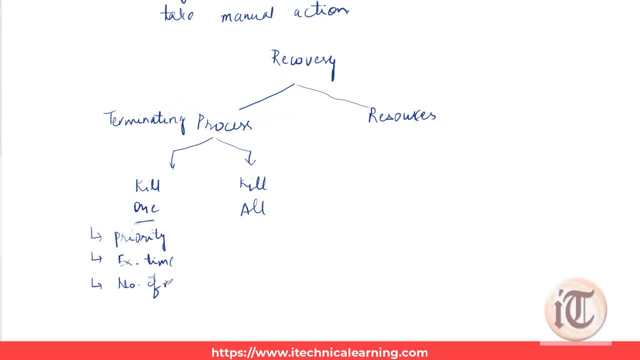 resources hold. okay, or maybe either it is interactive or batch. so there are so many criterias on which operating system identifies that which process is to be permitted next, and after the preemption of one process, the operating system tries to detect a deadlock in the system. that's why this approach is called as 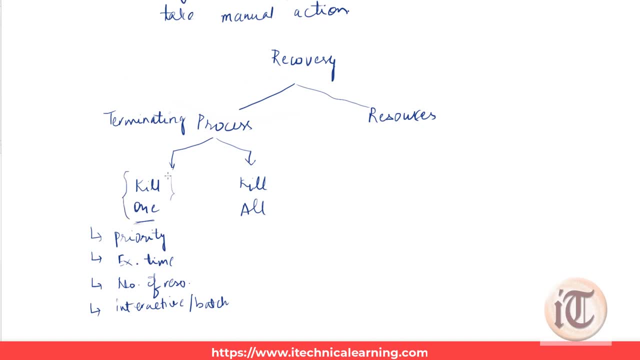 more conservative one and it takes time. the another approach, which is which is quite easy to perform, is called as kill all, that says, terminate all the processes that are involved in the deadlock. okay, this definitely solves the deadlock, but this approach is quite expensive. okay, this definitely solves the deadlock, but this approach is quite expensive. 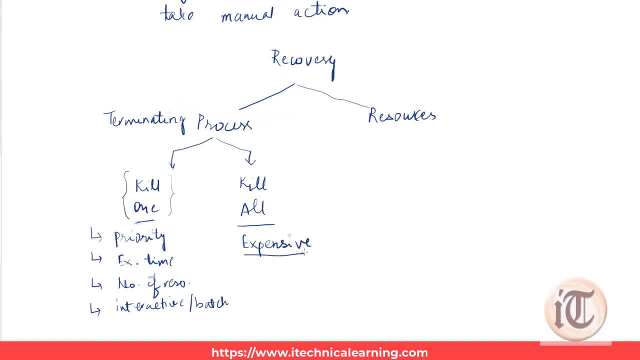 okay, this definitely solves the deadlock, but this approach is quite expensive. okay, by mean of saying expensive, I mean that suppose our system is executing ten processes at a time and if operating systems follows this strategy to overcome the deadlock, that is, kill all. so all these ten processes will be. 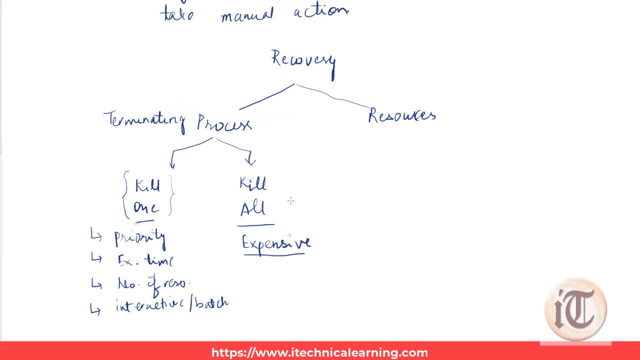 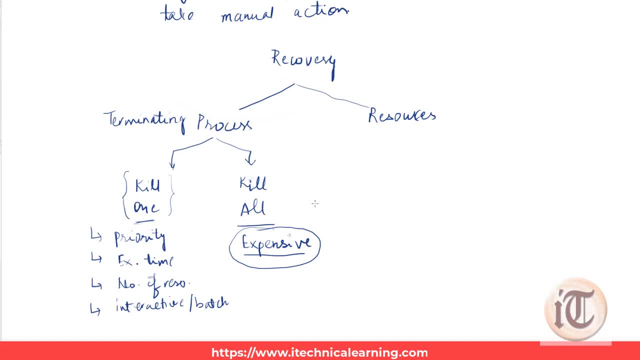 that's why I told that it is very expensive in terms of memory, in terms of execution time and so on. so this is the first approach for the from the recovery of deadlock that operating system takes. okay now, next approach: if operating system focuses on resources, okay, then we talk about the resource. 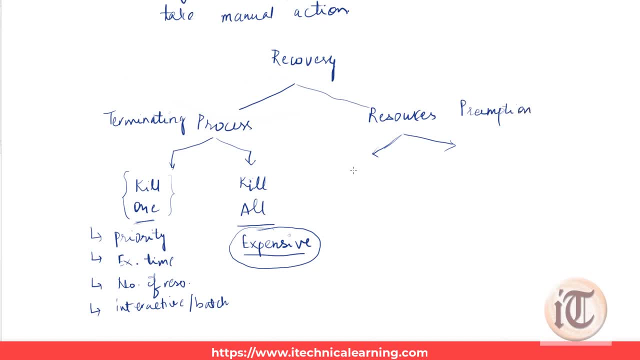 preemption, then this resource preemption can be done in major toolbox using of two ways. that is, first, select a victim. select a victim means that deciding which resources are to be preempted from which process that involves many of the same decision criterias as discussed here. okay, so in this we actually identify the resource that needs to be. 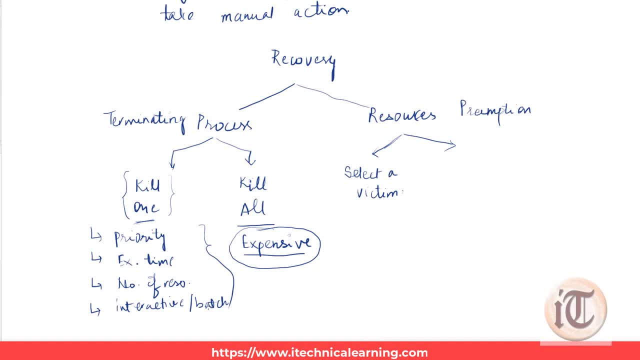 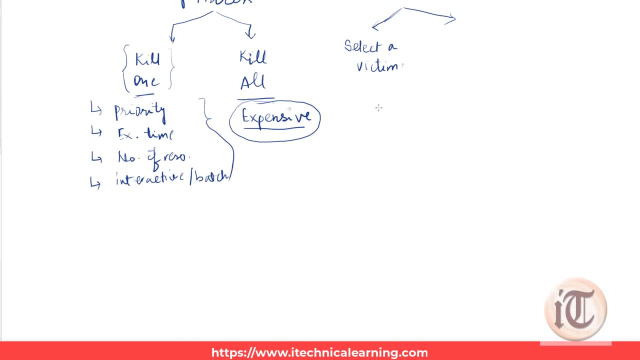 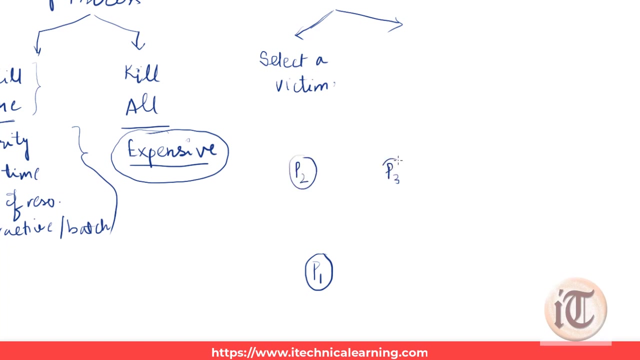 preempted, which is involved in the deadlock. okay, so if you take an example of this, select a victim. suppose we have a system which is having some processes. let us say this is process P 1. next we have say process P 2, then we have process P 3 and say we have one more process, that is P 4. 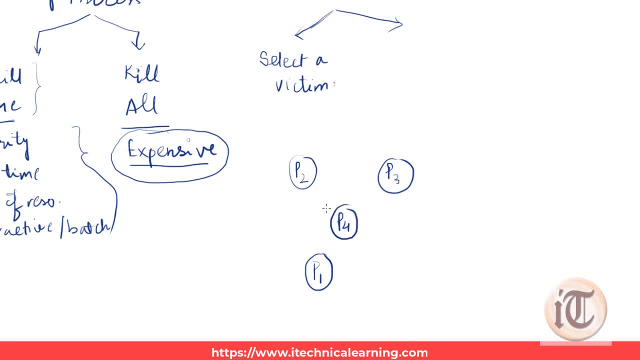 okay, now these processes are associated with particular resources. so let us say this is resource one or R 1 and this is resource two and this is resource say three. okay, and the interconnection of these process, two resources, as follows: that is, P 2 is waiting for R 1 and R 1. 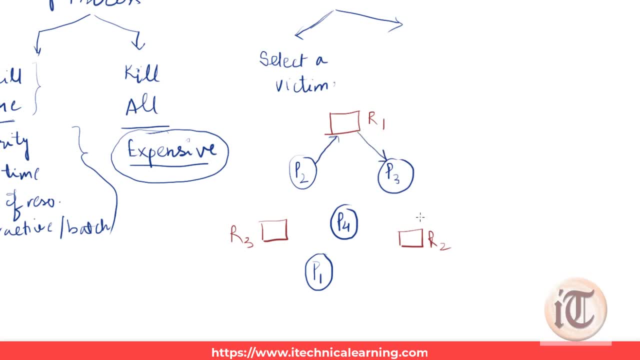 is allocated to P 3, P 3, P3 is waiting for R2 and this R2 is allocated to P4, P4 is waiting for R3 and this R3 is allocated to P2, and P1 is waiting for R3.. 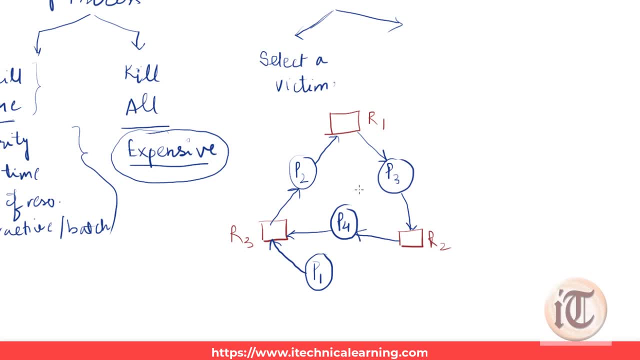 Now, as you can see, if you convert this into wait for graph, we will find a cycle. so this system is in deadlock. So to resolve it, what operating system does so? if you perform the resolution of it, it identifies any process and select as a victim. 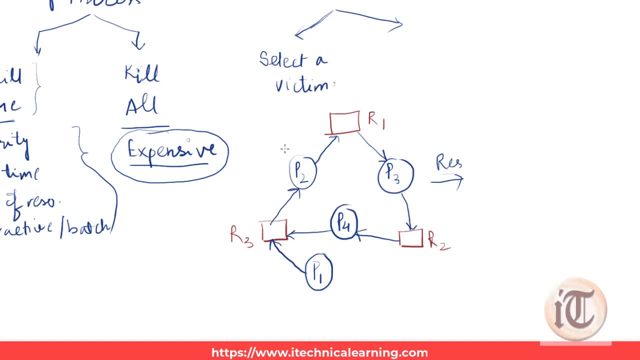 So if suppose operating system finds that P2 process is a victim on the basis of these particular criteria, that whether it is priority or execution time, or number of resources allocated, or interactive or batch, So it may happen that after particular moment or for the recovery process, the system state: 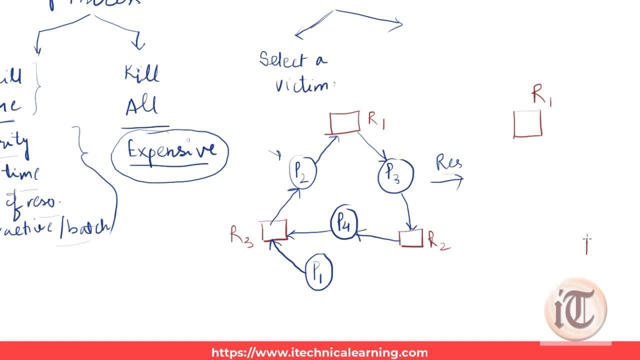 will now be something like: that is R1, then we have R2., Then we have P2.. Then we have P3.. Then we have P4., Then we have P5.. Then we have P6., Then we have R3, and if we talk about the processes, then we may have P3 and in between we have. 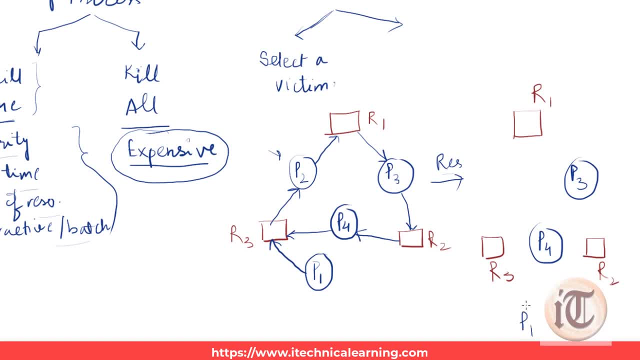 P4 and we have P1. okay, So we can see R1 is now located to P3, P3 is waiting for R2, R2 is allocated to P4, P4 is waiting for R3 and, as we have removed, 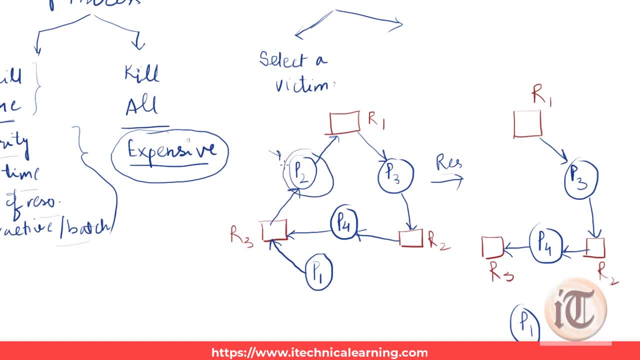 This P2 process after selecting it as a victim. So R3 resource, which was allocated previously to P2, is now free, So we can allocate this resource to the P1 process. okay, So we have broke the cycle here and we can see we have allocated R3 to P1 and P1 doesn't. 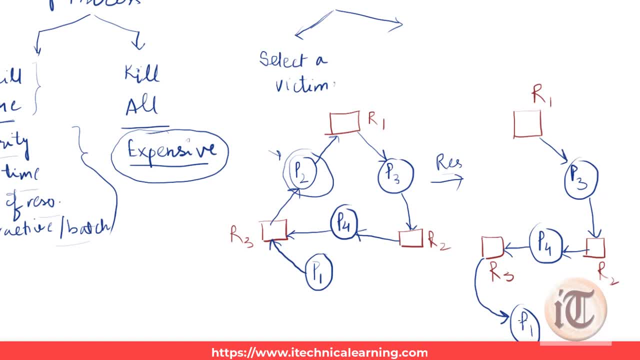 wait for any further resource. So P1 will be executed. after execution of P1, R3 will be free, So it can be allocated to P4, okay, and so on, so on, so on. So in this way We can break the deadlock or we can get the resolution from the deadlock situation. 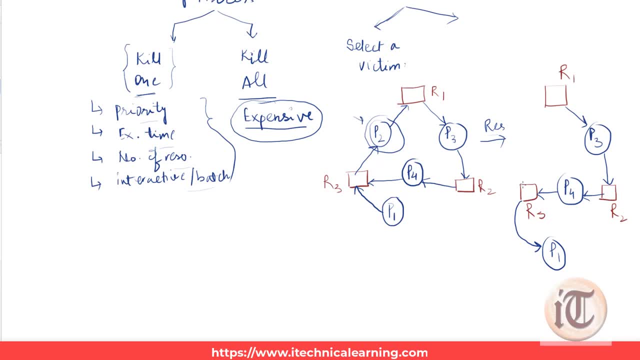 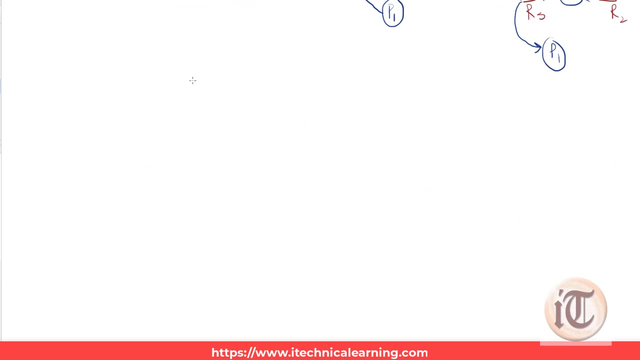 So this is- this is our first approach, which is called as selecting a victim- okay Now, if I continue with the second approach, then second approach says that rollback- okay Now. rollback means if you are dealing with the rollback, Then it is the callback. So this is the concept, something like this. 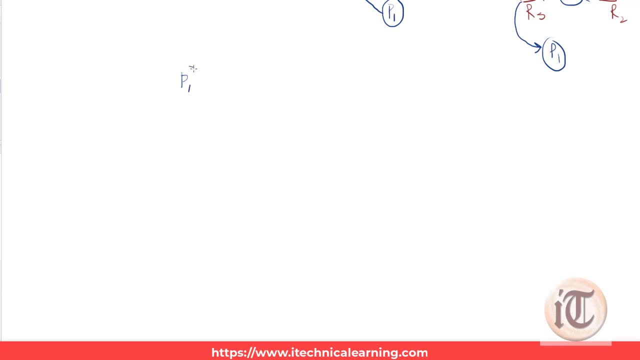 Suppose P1 is a process which is executing Which has the execution time of, say it wants total 10 milliseconds to execute. okay, And suppose it has executed 4 milliseconds till now and after that it has got involved in some deadlock situation which is unwanted situation. okay, 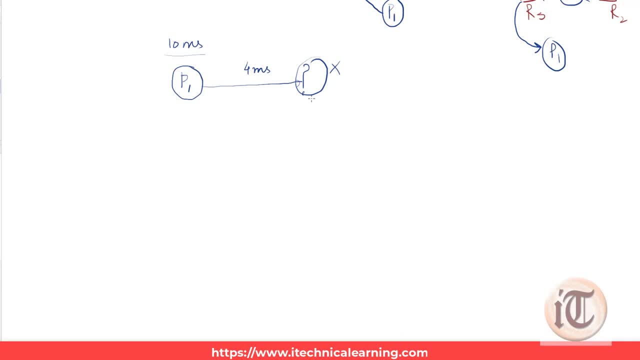 So what operating system can do that? to resolve a deadlock, It can perform a rollback. Set the rat, okay. and to perform a rollback the operating system has to find a safe state in which the process was previously designated. okay, but you can see, if we have one process, then we can add. an operating system can identify. 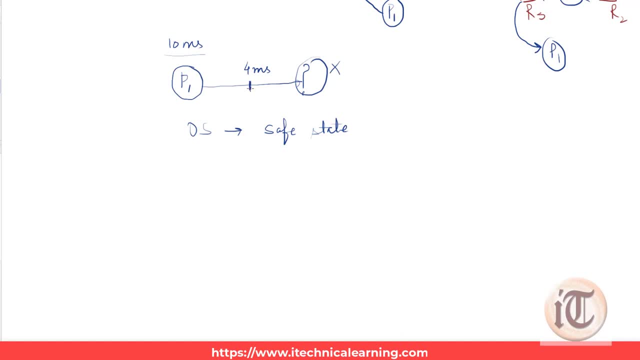 that suppose this one was the previous safe state that till now there was not no symptom of deadlock. so we can roll back from here to here. okay. but if we have multiple processes, say, operating system is executing 50 processes at a time. so in that particular situation it is very tedious process for an operating 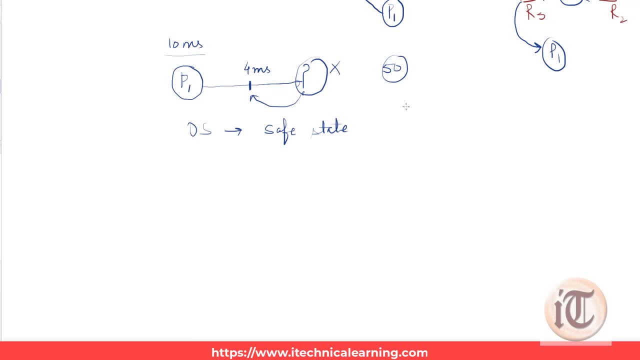 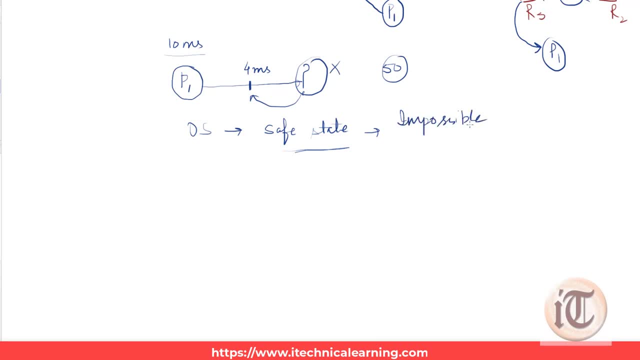 okay. or we can say it is almost impossible to find such safe state. so the ideal situation for rollback is that this process, that is P 1, will be rolled back to its initial state. okay, so suppose if we have P 1, we have P 2, we have P 3, we have P 4, we have multiple processes. so 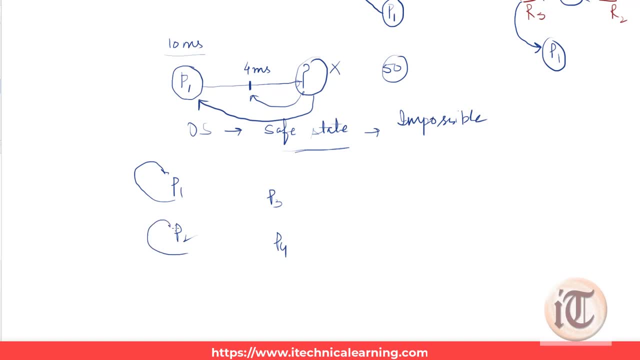 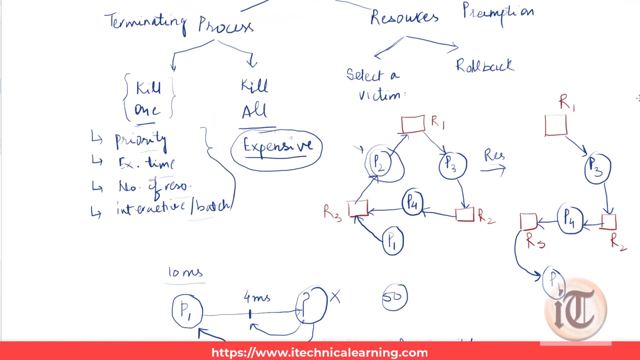 all processes will be rolled back to their original state, that is, or initial state, that is 0, okay, so this is the only safe rollback situation that operating system can guarantee. guarantee that is: that means the abort the process, or we can write it as abort the process. abort means terminated and abort it to the starting point. okay, but 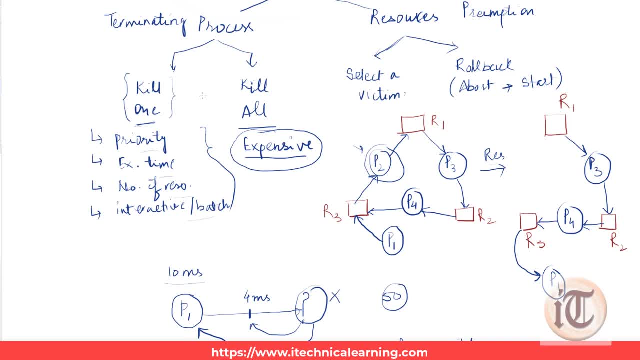 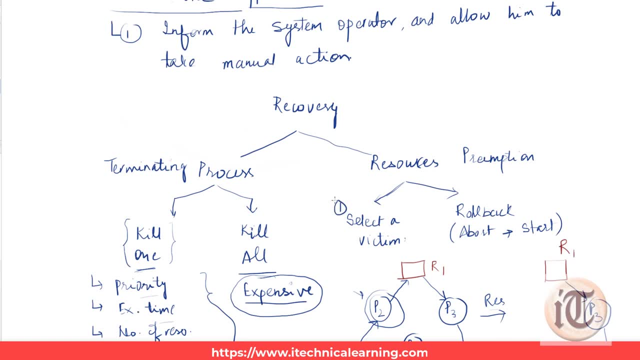 there is one situation or one issue that this resource prevention has to deal, because we are talking about the selecting a victim or rollback. so in both the situations, we have to deal with this resource prevention because we are talking about the selecting a victim or rollback. so, in both the situations, the resource prevention.